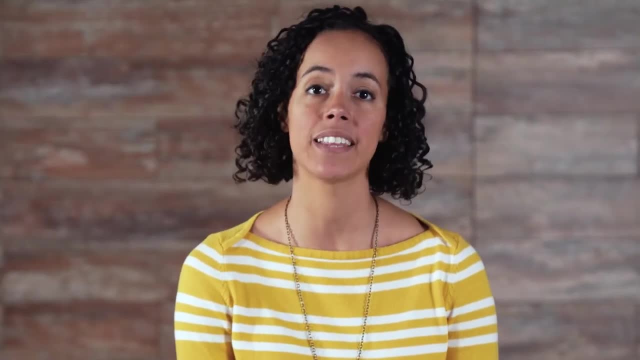 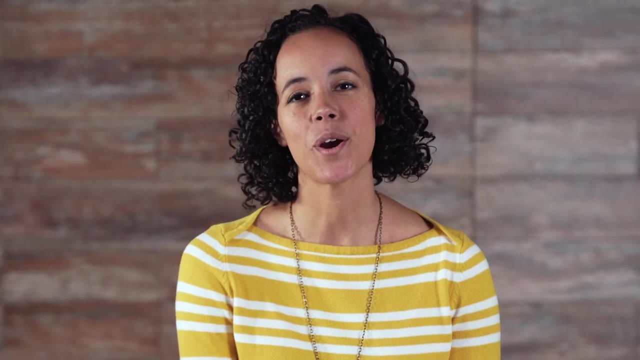 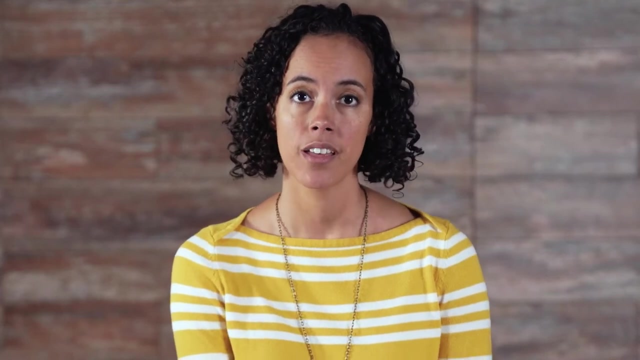 Hi and welcome to this video covering the least common multiple and the greatest common factor. As you know, there are times when we have to algebraically adjust how a number or an equation appears in order to proceed with our math work. We can use the greatest common factor and the 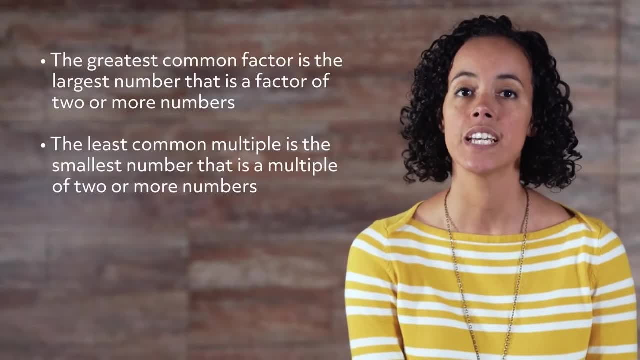 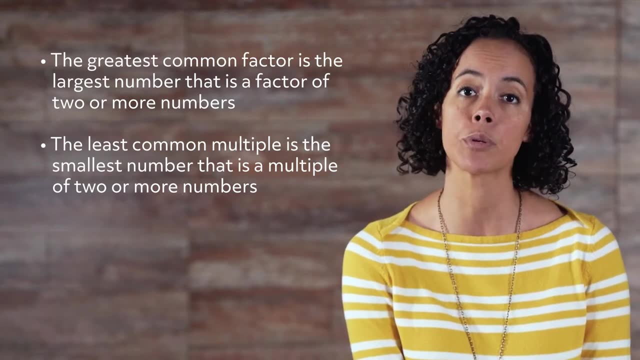 least common multiple. to do this, The greatest common factor is the largest number, that is, a factor of two or more numbers, and the least common multiple is the smallest number, that is a multiple of two or more numbers. To see how these concepts are useful, let's look at adding. 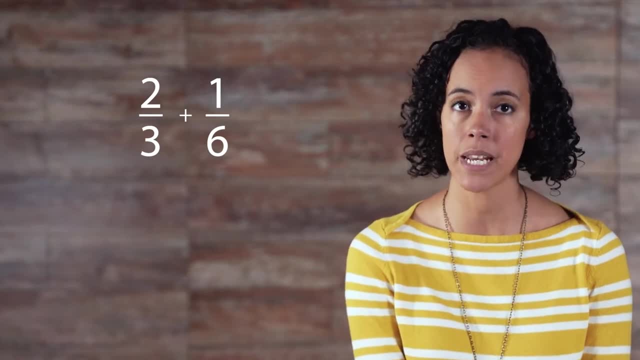 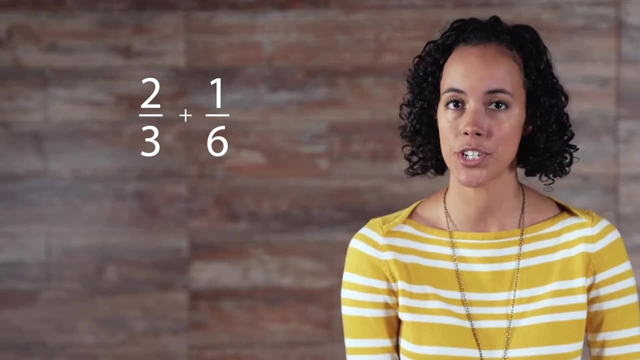 fractions. Before we can add fractions, we have to make sure the denominators are the same. by creating an equivalent fraction, In this example, the least common multiple of 3 and 6 must be determined. In other words, what is the smallest number that both 3 and 6 can divide into evenly? 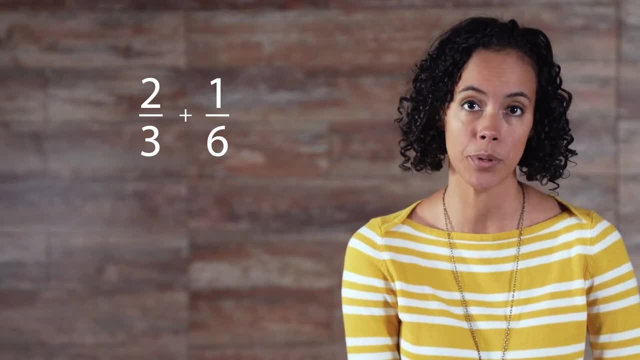 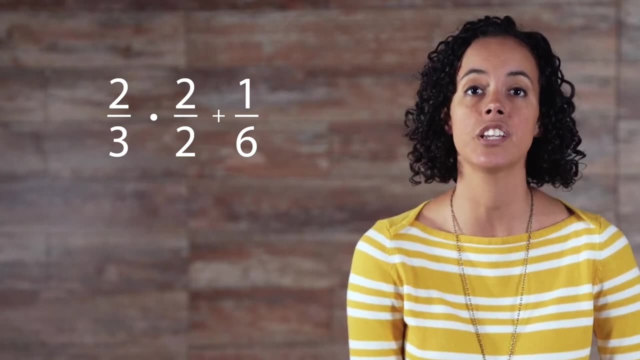 With a little thought, we realize that 6 is the least common multiple, Because 6 divided by 3 is 2, and 6 divided by 6 is 1.. The fraction 2 over 3, is then adjusted to the equivalent fraction 4 over 6, by multiplying both the numerator and denominator. 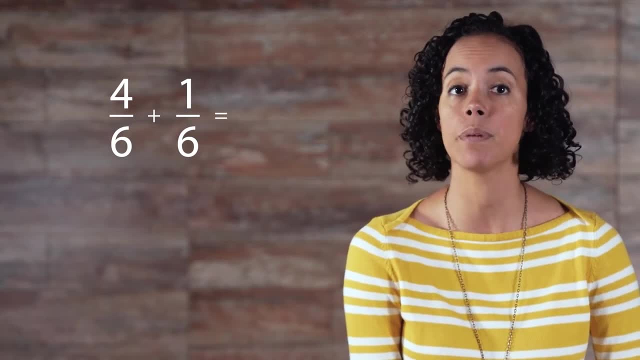 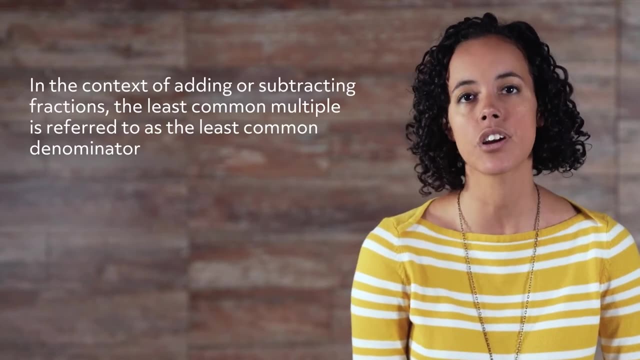 by 2.. Now the two fractions with common denominators can be added for a final value of 5 over 6.. In the context of adding or subtracting fractions, the least common multiple is referred to as the least common denominator. In general, you need to determine a number larger than or: 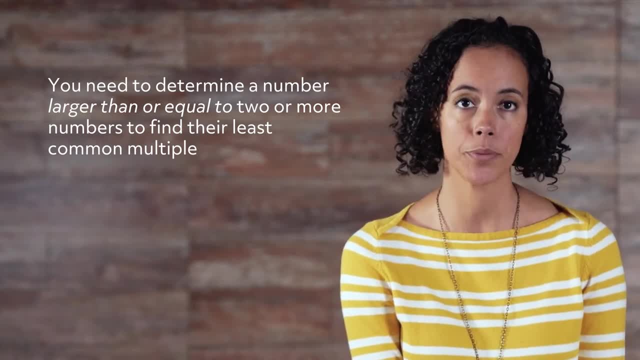 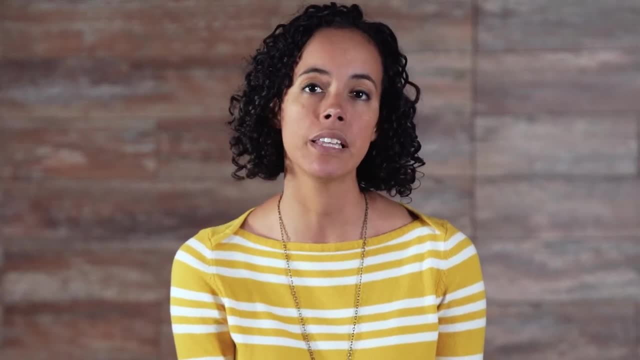 equal to the least common denominator. In general, you need to determine a number larger than or equal to 2 or more numbers to find their least common multiple. It's important to note that there is more than one way to determine the least common multiple. One way is to simply list all the 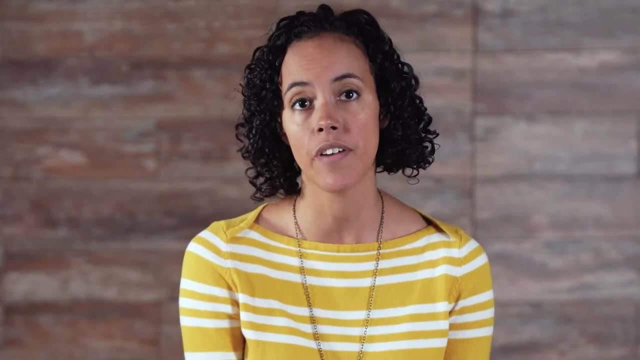 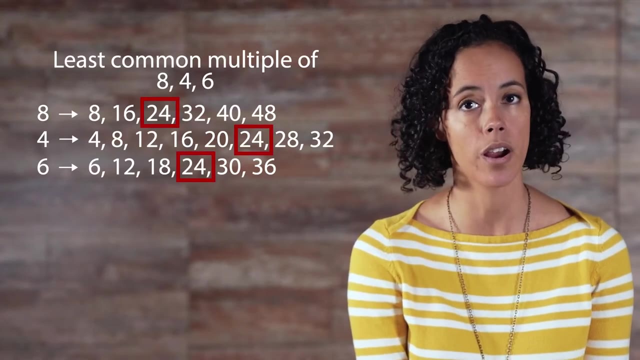 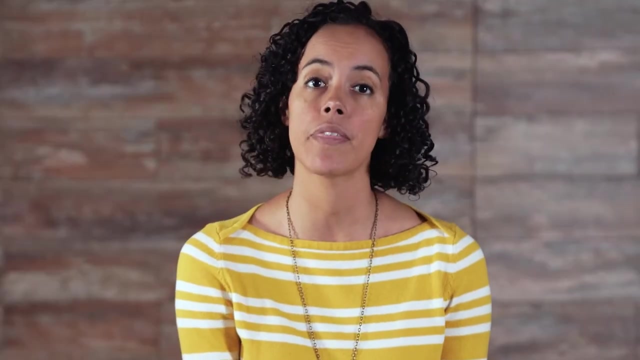 multiples of the values in question and select the smallest shared value, as seen here. This illustrates that the least common multiple of 8,, 4, and 6 is 24, because it is the smallest number that 8,, 4, and 6 can all divide into evenly. Another common method involves the prime factor. 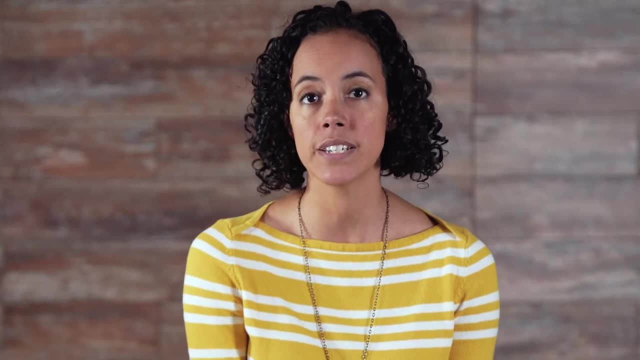 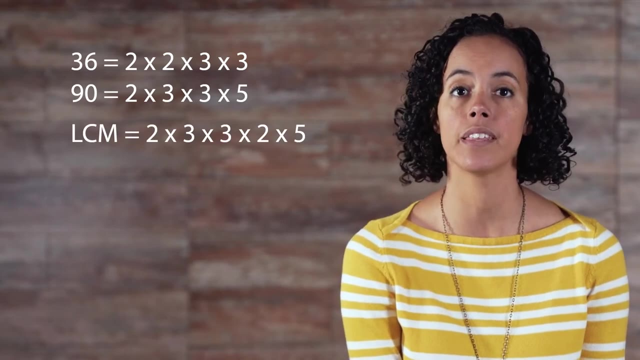 factorization of each value. Remember a prime number is only divisible by 1 in itself. Once the prime factors are determined, list the shared factors once and then multiply them by the other remaining prime factors. The result is the least common multiple, The least common multiple can.